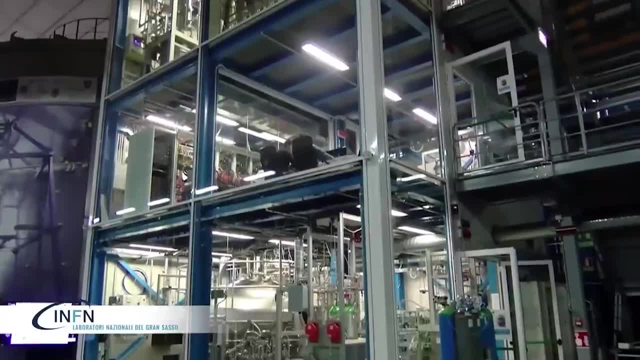 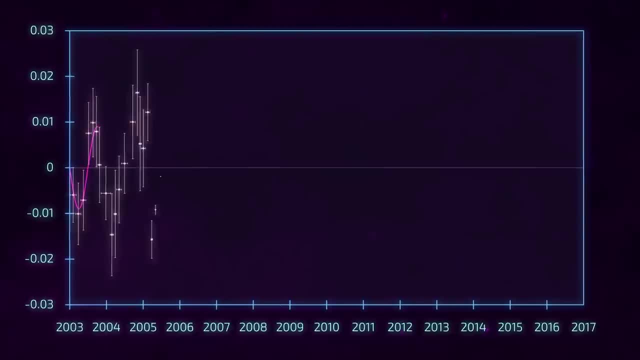 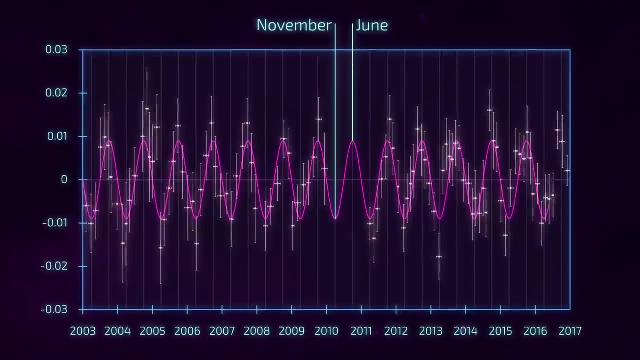 It's been collecting data for around 20 years and every year it sees the same peculiar results. The rate of detections increases to a peak in time. It starts in June and then decreases to a minimum in November. Some scientists think this could be the first direct evidence of dark matter. 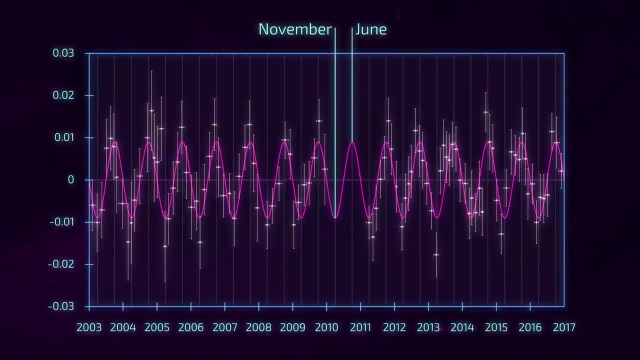 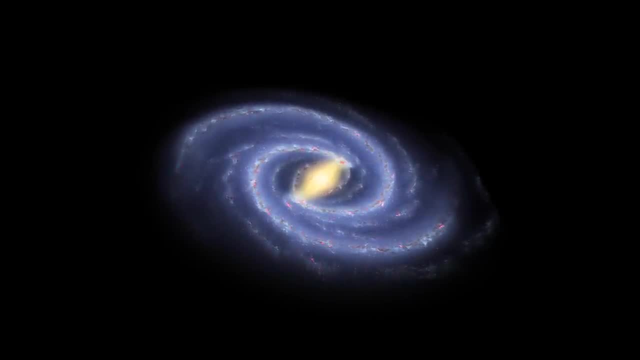 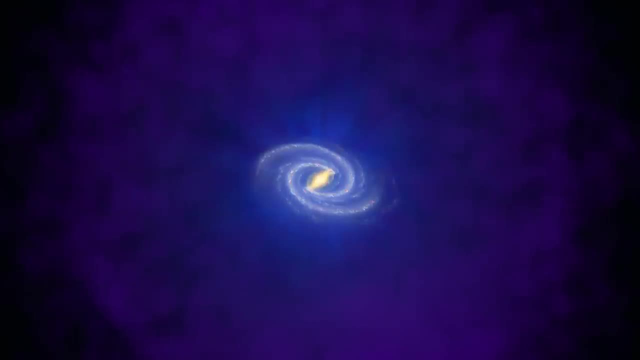 But why would dark matter create a periodic, annual signal? Well, this is our galaxy, or at least what it looks like with visible light. Astronomers suspect it is surrounded and permeated by a huge sphere of dark matter, Invisible particles Flipping around, all in random directions. 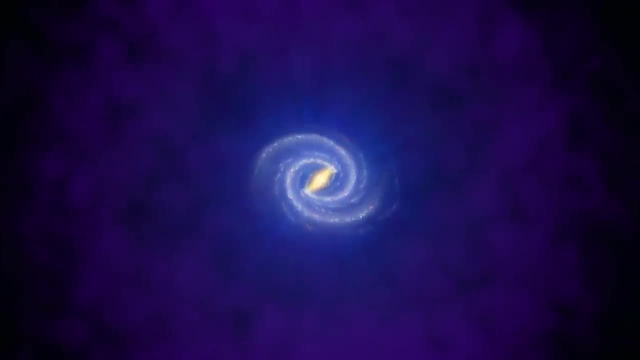 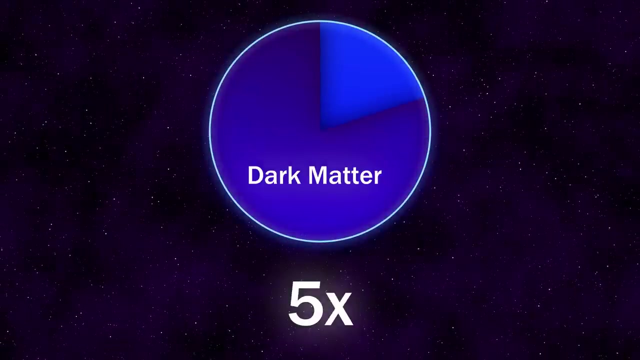 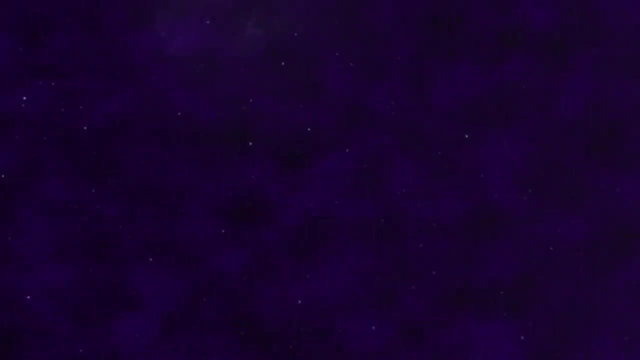 According to most theories, dark matter doesn't interact with anything, including itself, except through gravity. We think there should be five times as much dark matter as there is ordinary matter. Now our solar system is moving around the galaxy at 220 kilometers per second. 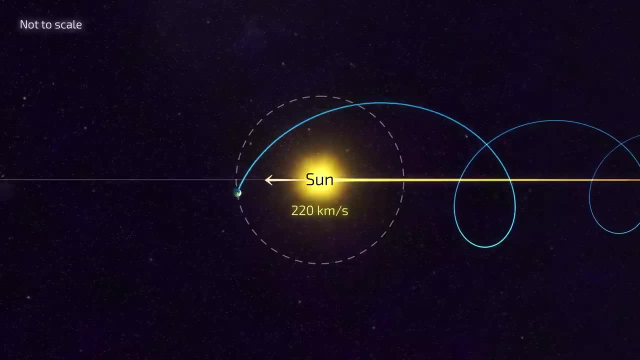 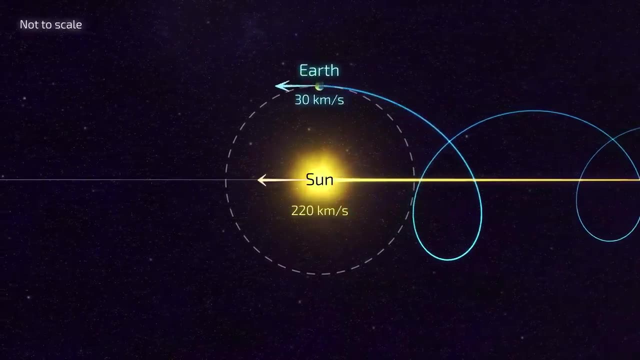 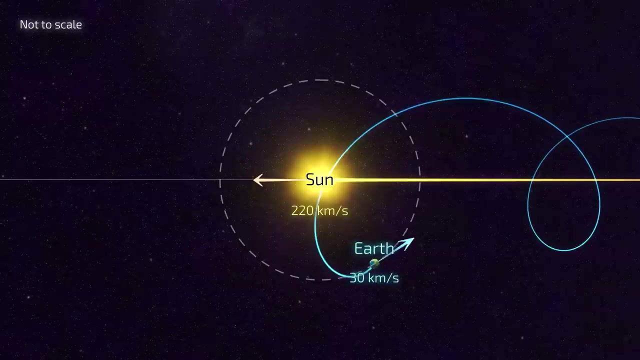 That means we're also moving through dark matter at this rate, Except Earth orbits the Sun at 30 kilometers a second. So for half the year we're moving with the Sun going faster through dark matter And the other half the year we're moving in the opposite direction, so going slower through dark matter. 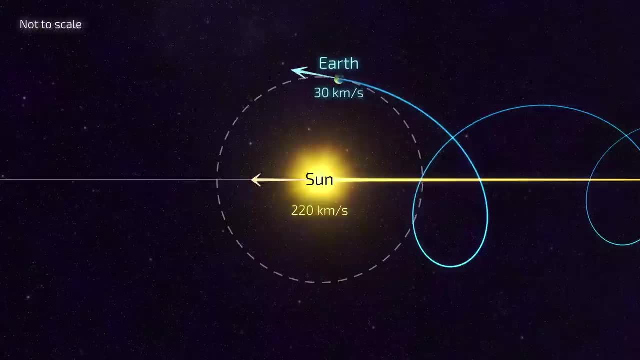 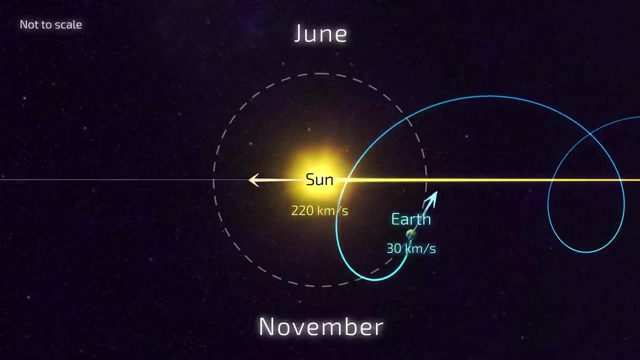 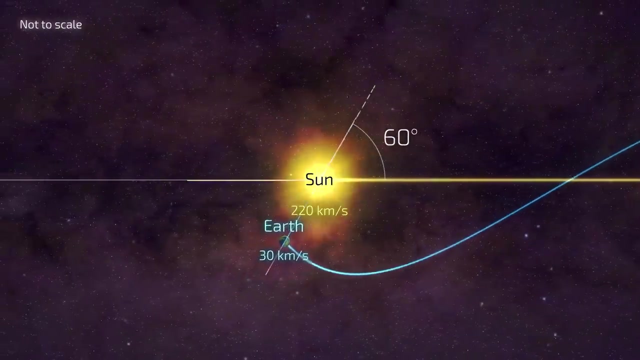 And the idea is we encounter more dark matter when we're moving through it fastest, which happens to be in June, and less of it when we're moving slowest, which happens in November. The actual geometry is a little more complicated. The solar system is tilted at 60 degrees relative to the plane of the galaxy. 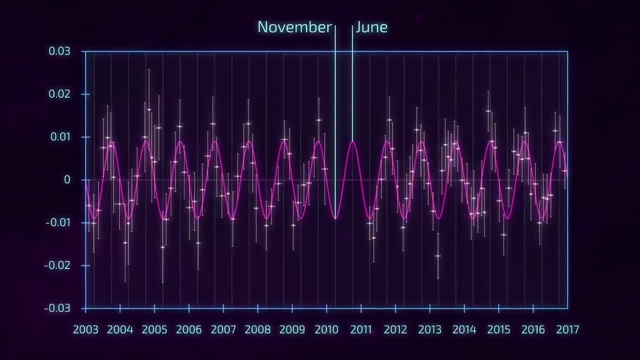 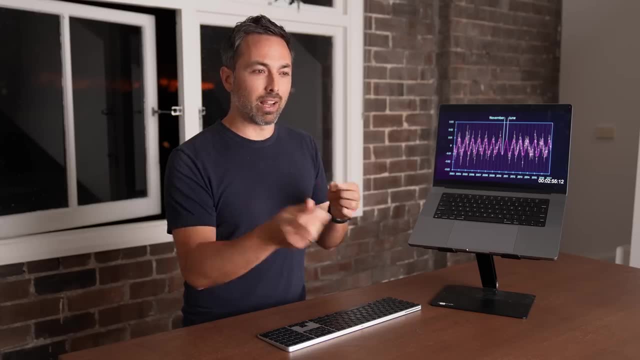 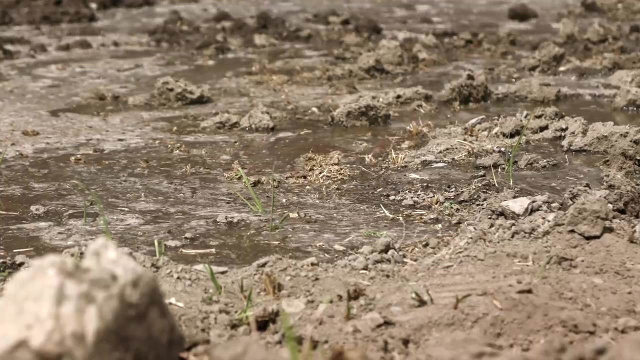 But the idea still works. So the signal observed at Dama Libra may be due to this motion through dark matter, Or it might not be due to dark matter at all. It could just be something mundane like the temperature, humidity, moisture in the soil, the snow on the mountain. 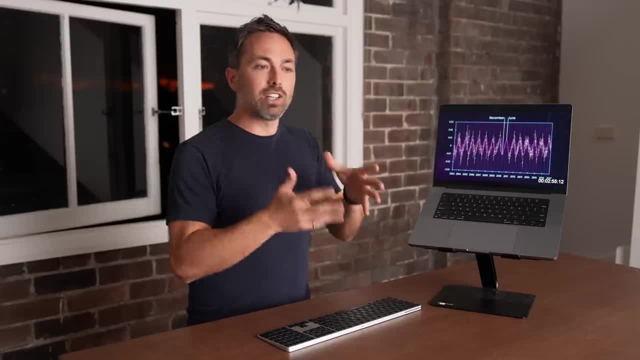 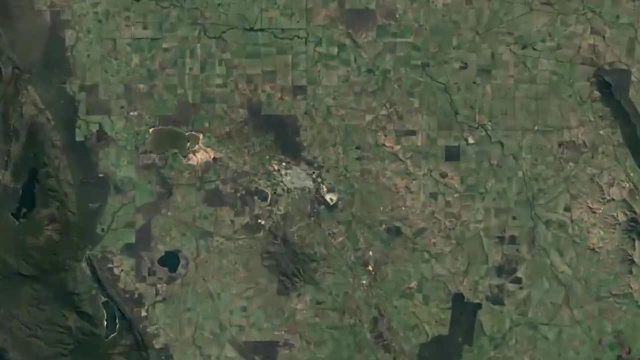 or the number of tourists in the galaxy. All of these things fluctuate with a period of one year, And that is why they're going to build an almost identical experiment in the southern hemisphere, down the bottom of this gold mine outside of Melbourne. 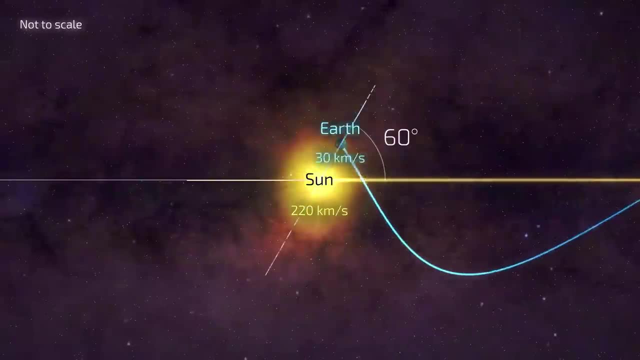 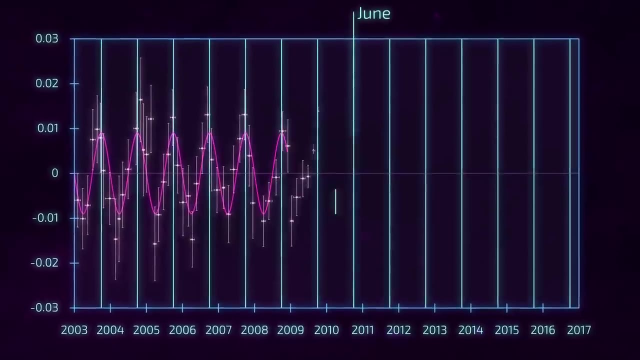 Because there the seasons are reversed, but our motion through dark matter is still the same. So if we see the same signal, it's pretty strong evidence for the existence of dark matter. One of the big problems that Dama Libra has is that there are other very similar experiments. 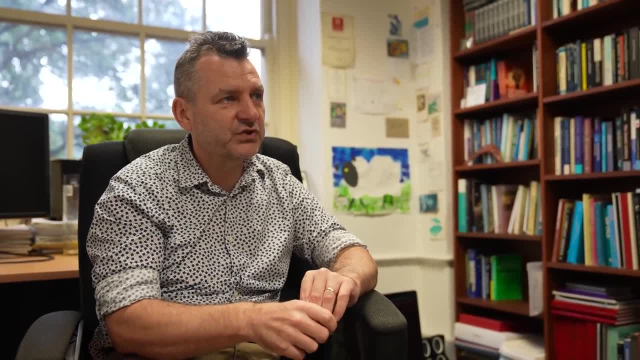 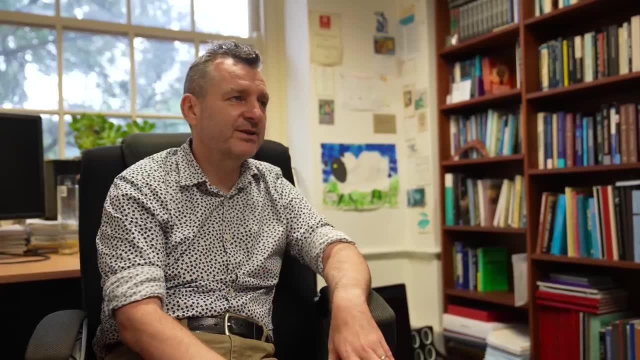 that don't see anything And this has led to, you know, a lot of uncertainty about: is the Dama Libra signal really dark matter? So, yeah, you know, we don't know right, The favorite thing in science. 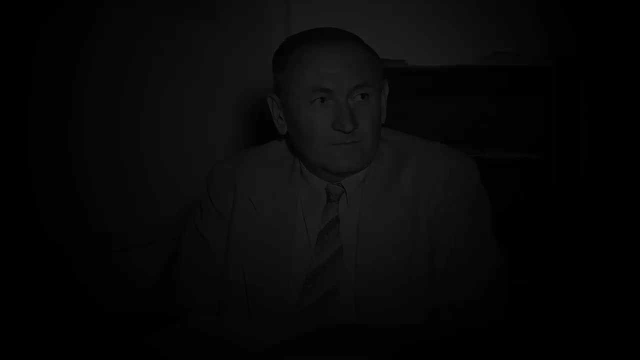 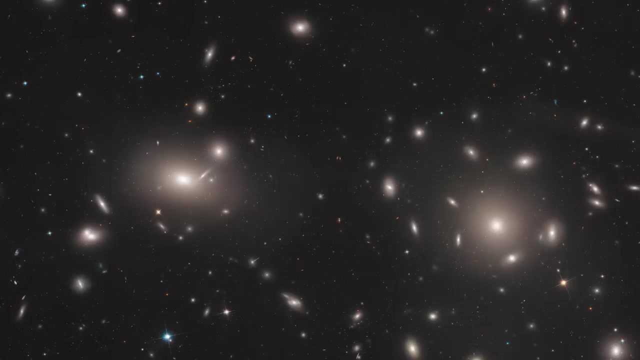 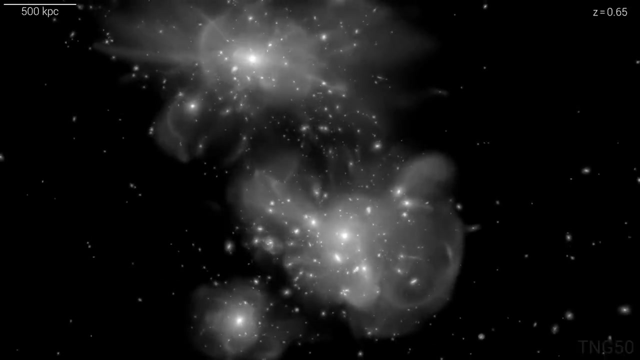 But why do we think dark matter exists in the first place? In 1933, Swiss astronomer Fritz Zwicky was studying the Coma Cluster, a collection of more than a thousand galaxies. These galaxies are gravitationally bound together, So they all orbit around their collective center of mass. 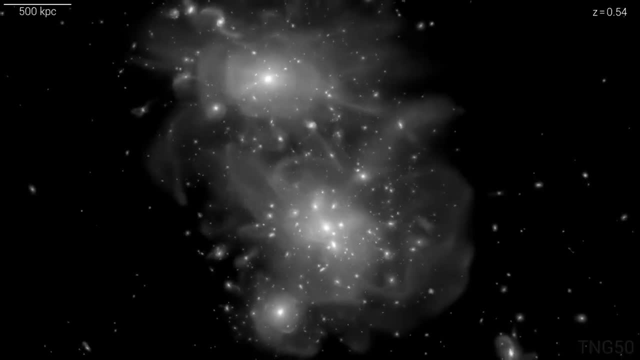 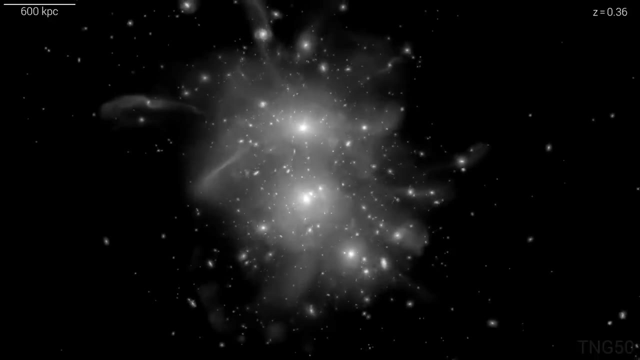 Zwicky measured the orbital speeds of these galaxies and found that some were moving way faster than he expected. It was as if there was a lot more matter in the cluster than he could see, pulling everything inwards. So he proposed the existence of invisible matter. 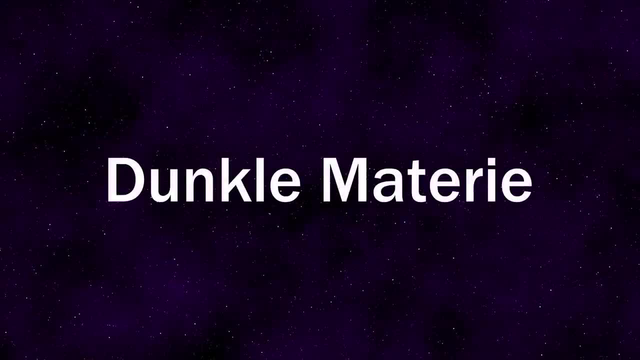 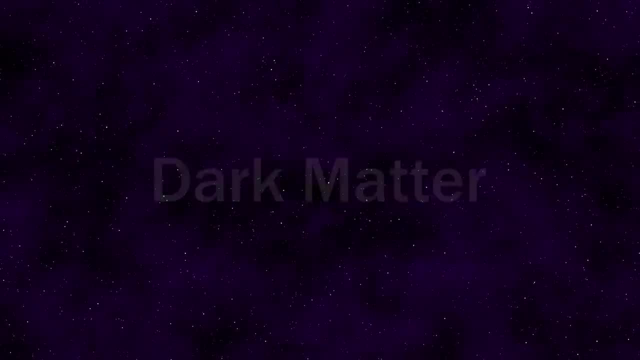 which he called dunkelmaterie, the origin of the term dark matter. No one really took this idea seriously, but 40 years later dark matter turned up again. Vera Rubin and Kent Ford observed the motion of stars in the Andromeda galaxy. 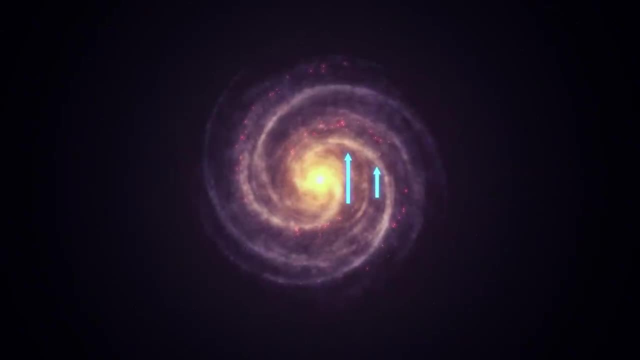 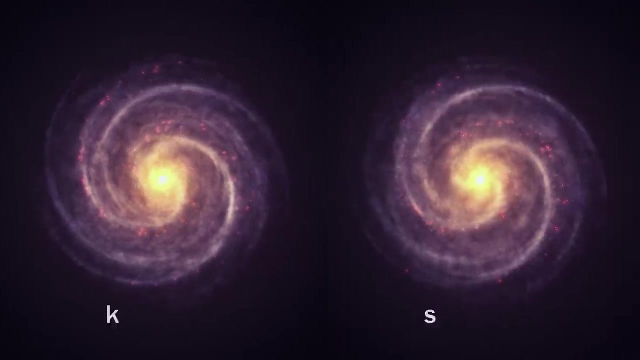 and they expected that the further out from the center you go, the slower the stars would be orbiting. But this is not what they found. The rotational velocity stays almost constant with increasing distance from the center, Without additional mass in the galaxy to pull those stars in. 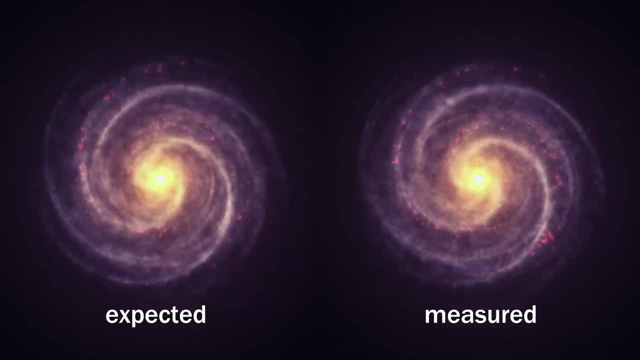 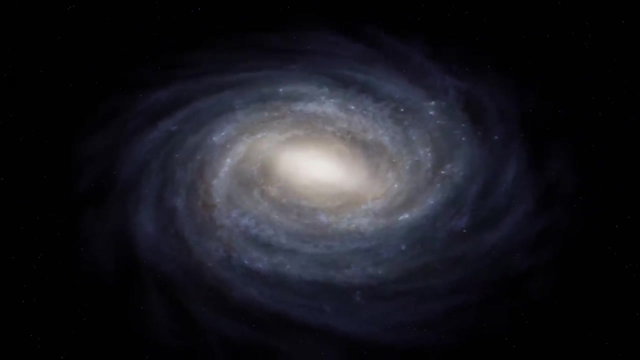 they should be flung off into space. The result was the same in other galaxies. Using radio telescopes, Albert Bosma and others measured hydrogen gas even further out from a galaxy's center, But the rotational velocity still stayed constant. One way to explain this is to posit the existence of matter we can't see. 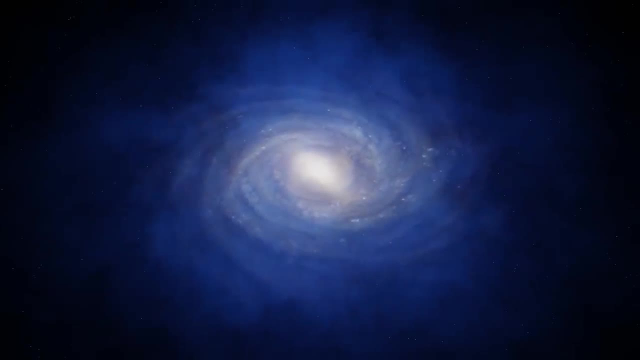 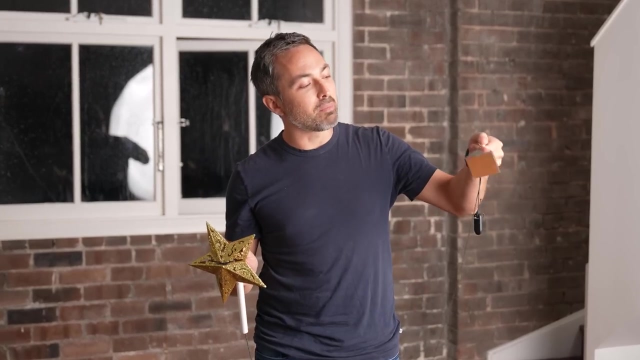 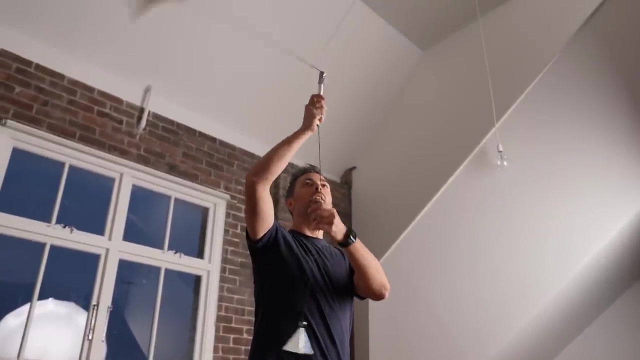 dark matter which holds all these galaxies together. So let's say you have a star and this represents the mass of everything in the center of the galaxy that's pulling the star in. The star can maintain a stable orbit if its centripetal force. 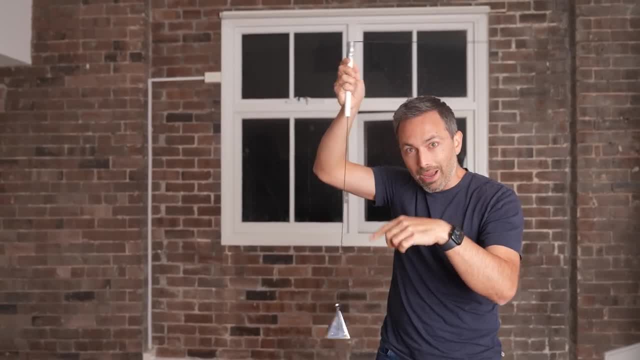 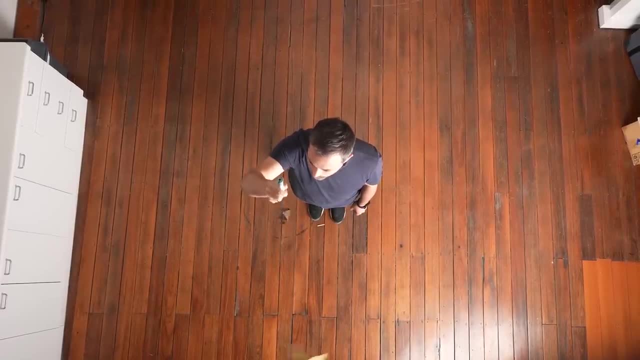 is equal to the gravitational attraction to all the mass in the rest of the galaxy, And so you can see that at about a distance of one meter, this is the speed of the orbit. Okay, but what happens if we add some dark matter? 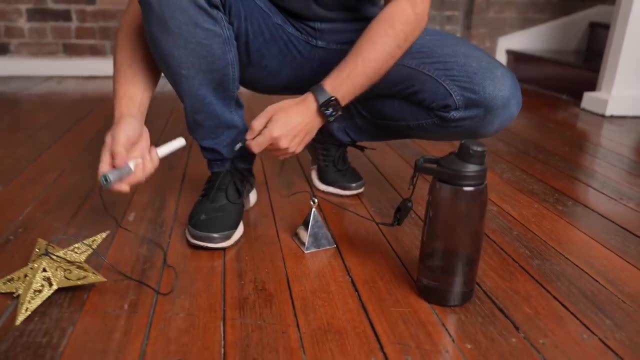 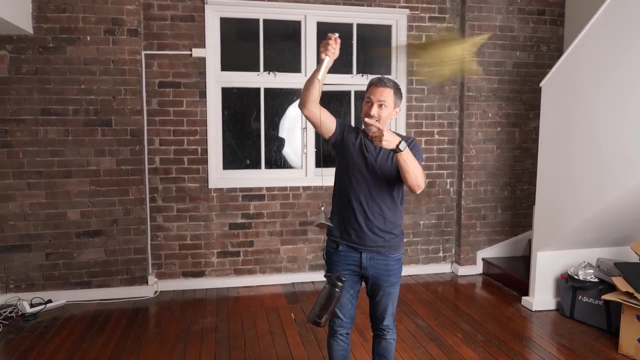 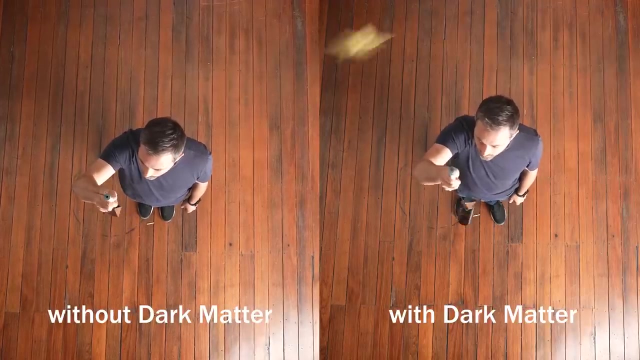 So this water bottle represents the matter we can't see. Now there is more mass pulling this star into the middle, which means at the same orbit. it can now go much faster and in fact it must go faster to maintain that orbit. 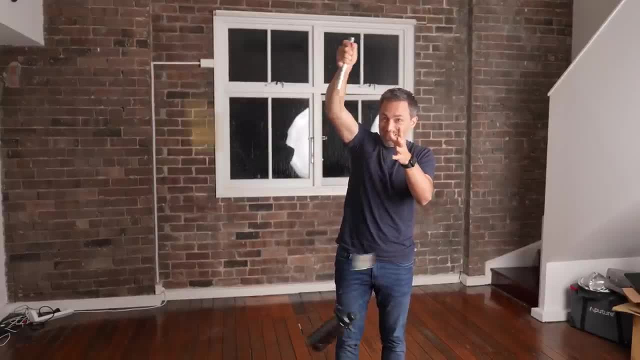 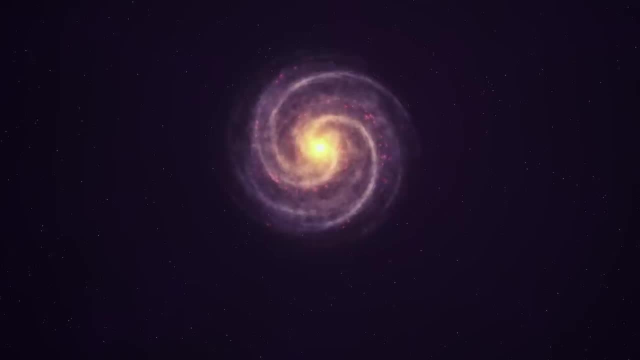 And this explains the observation. This is what we see By looking at the rotation speeds of stars. scientists estimate that about 85% of the mass of a galaxy is dark matter. But there's another way to explain these observations Without invoking dark matter. 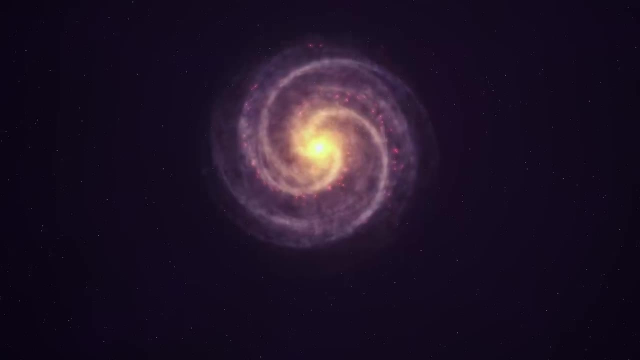 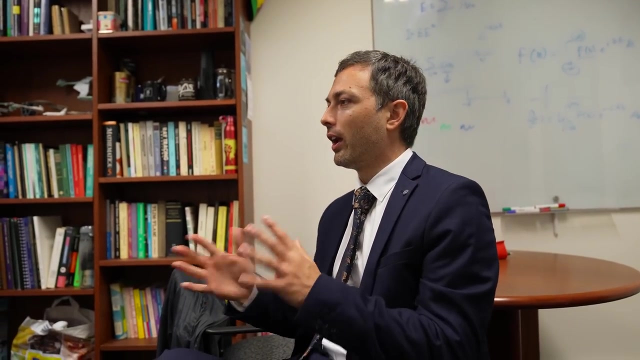 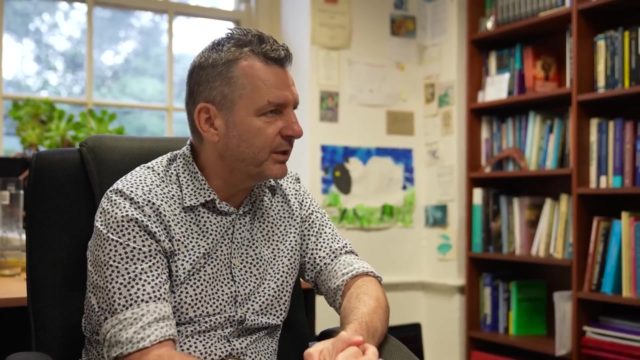 And that is to modify our theory of gravity. What's the supporting evidence for thinking that the particle idea is totally misguided and that we should actually be looking at a revised theory of gravity? You can either invoke something we can't see or you just say: well, the universe is what we can see. 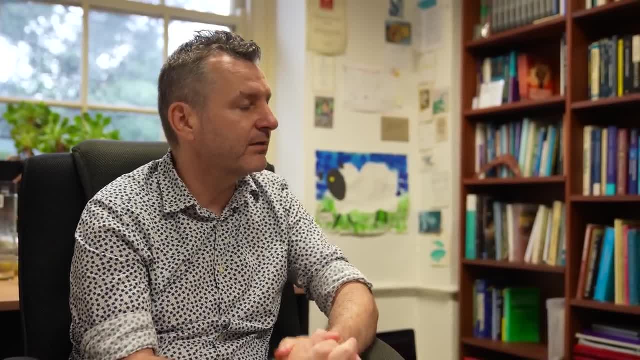 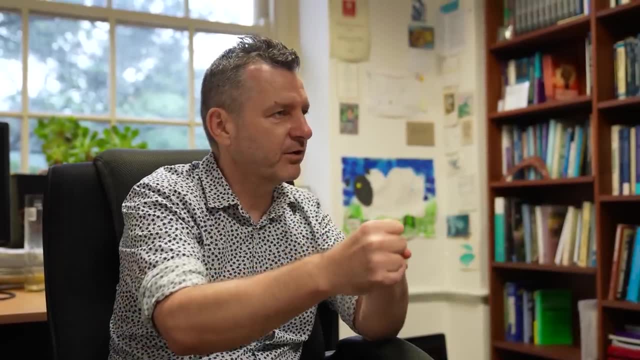 and we need a way to explain what's going on out there, And the only way we can do that is by modifying the laws of physics. So when you look at the outskirts of galaxies, they've got a lot of centripetal acceleration. 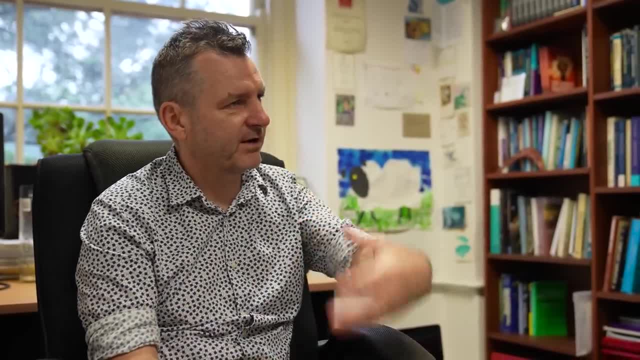 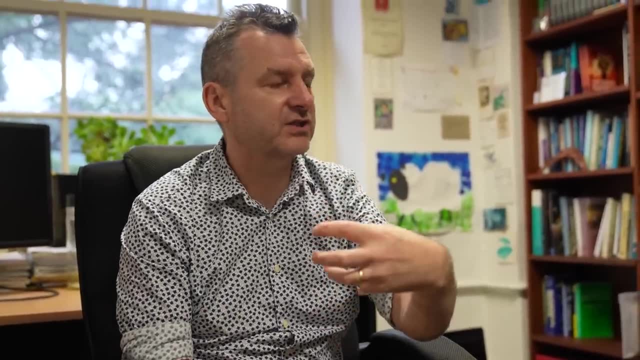 Dark matter says well, that centripetal acceleration is due to the gravitational effect of dark matter, Whereas people like Mond will say, no, that's centripetal acceleration, that's just the fact that it's now reached this floor and can't get any lower. 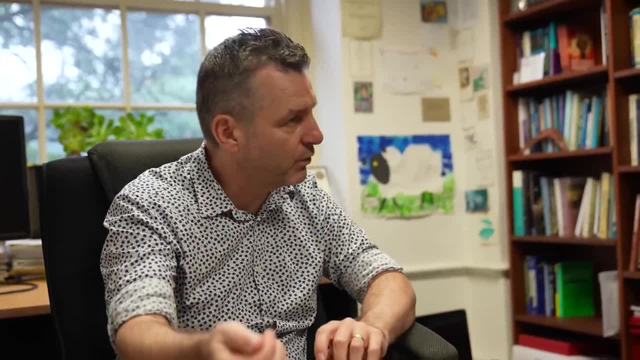 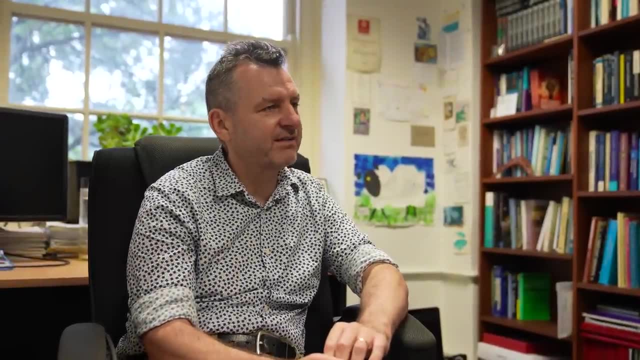 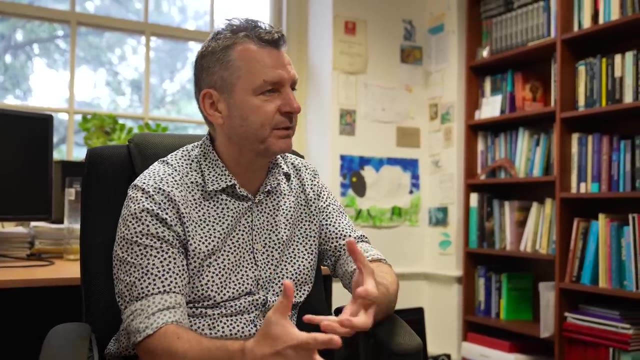 So they're saying that there's not additional force due to dark matter, but there's a limit to how low the acceleration could go. I think the consensus is hugely in favour of it being a physical substance, In that it just seems reasonable that there could be other particles out there. 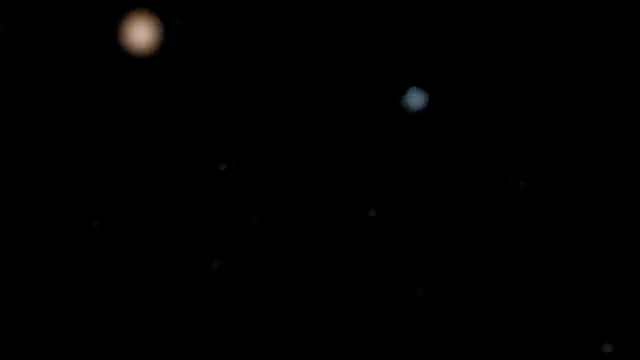 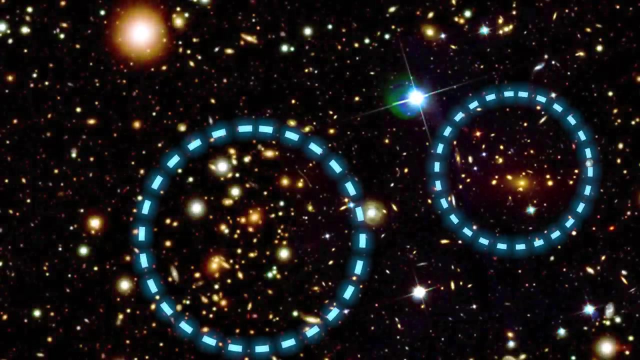 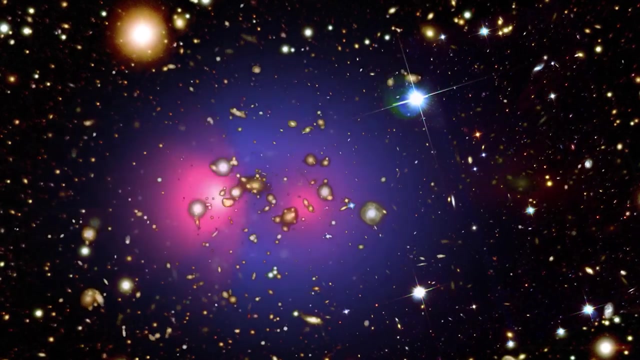 that we haven't seen yet And there's more evidence. This is the Bullet Cluster, a site where two clusters of galaxies collided. Most of the ordinary mass of these clusters is in the interstellar gas, And when the collision occurred, the interstellar gas interacted. 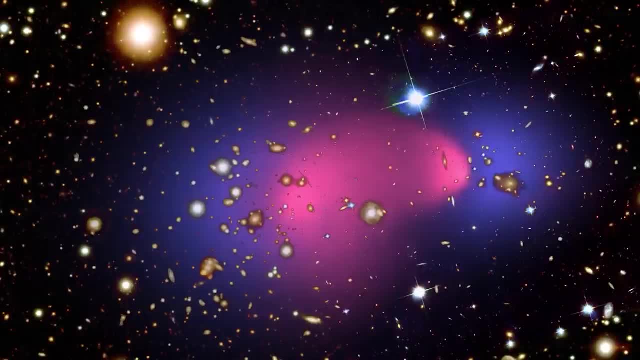 heated up and slowed down. So you'd expect that most of the mass of the Bullet Cluster would be in the middle, where all of this gas is. But if you use gravitational lensing- the way that gravity bends light- you can actually measure where most of the mass. 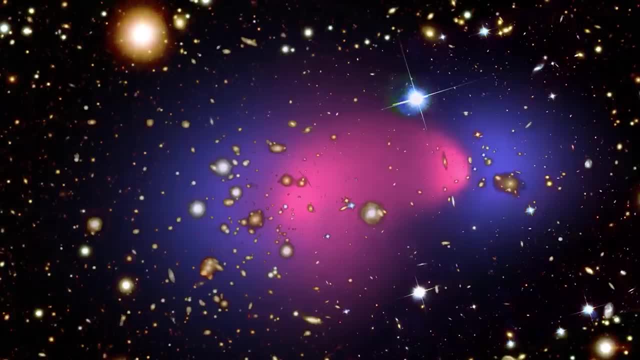 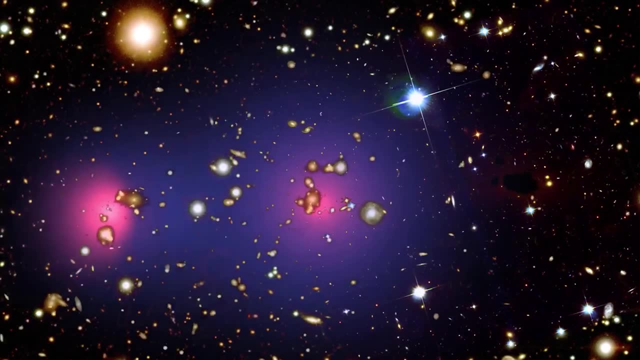 in this picture is And it isn't in the middle, It's actually on either side. So the best way to explain this is that when the clusters collided, all that gas got stuck in the middle, but the dark matter passed right through. 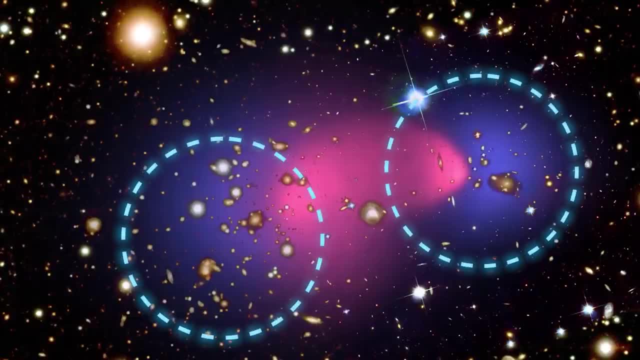 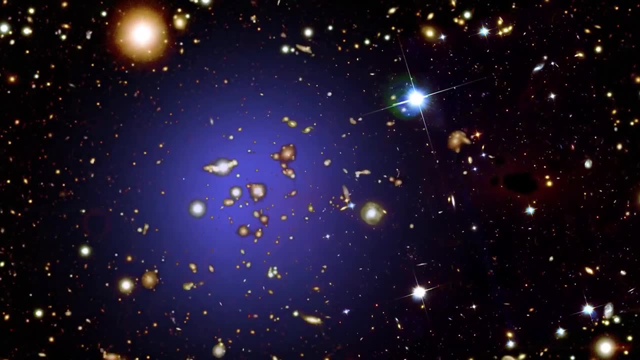 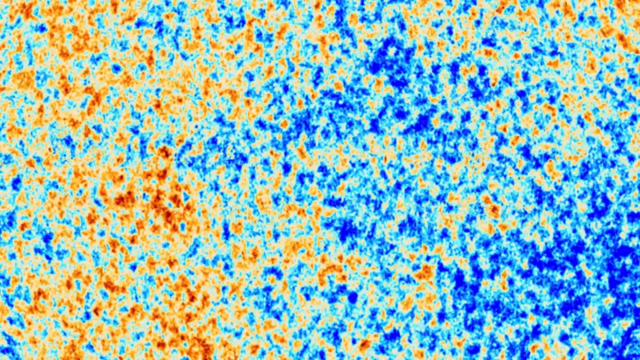 creating the most gravitational lensing where we can see the least ordinary matter. Even more evidence for dark matter comes from the oldest light in the universe. 380,000 years after the Big Bang, light could finally travel through the universe unimpeded. 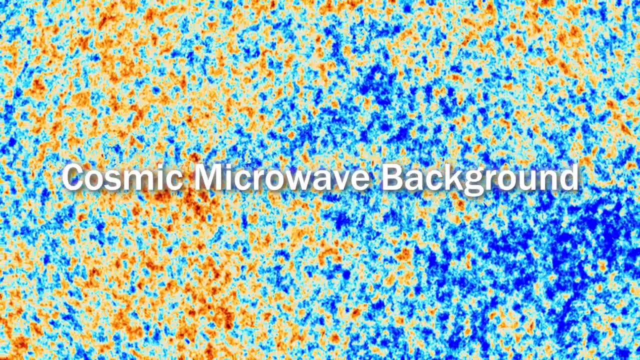 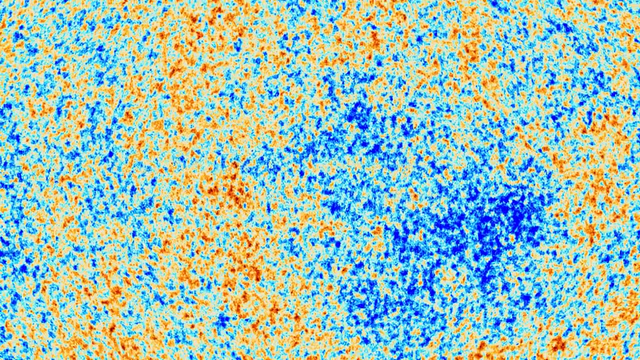 And this is what we see as the Cosmic Microwave Background, or CMB. The red spots show where the early universe was a little hotter and the blue spots show where it was a little cooler. These temperature differences were tiny, just .01%. 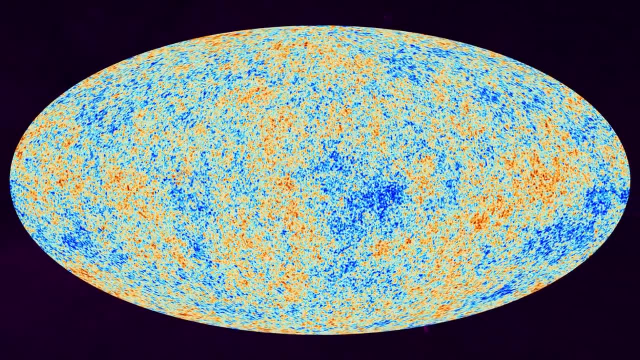 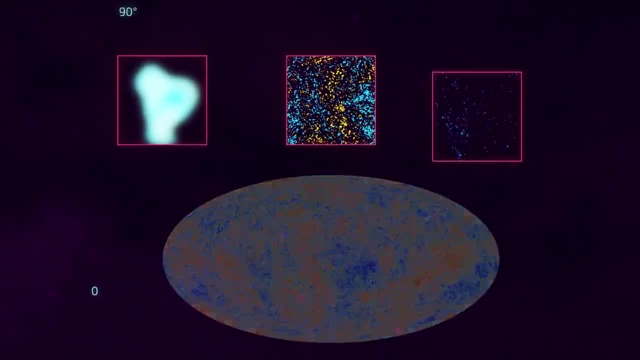 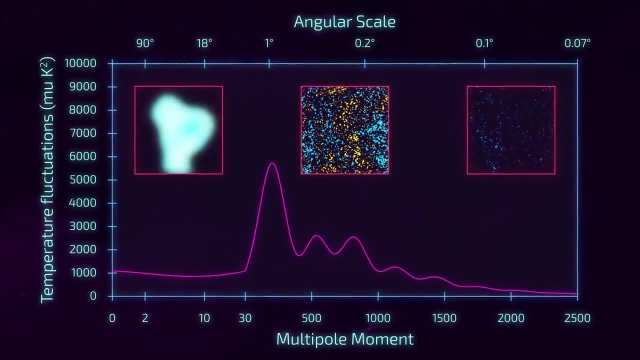 but they are there, And you can turn this picture into a graph by counting up how many blobs there are of different sizes. So there's the most common size blob which results in this peak, But there are also other common size blobs, and so you get these other peaks. 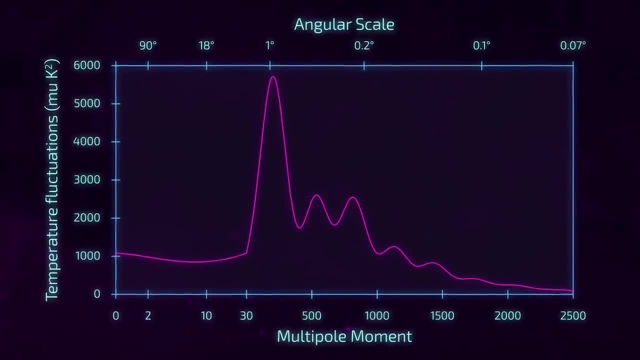 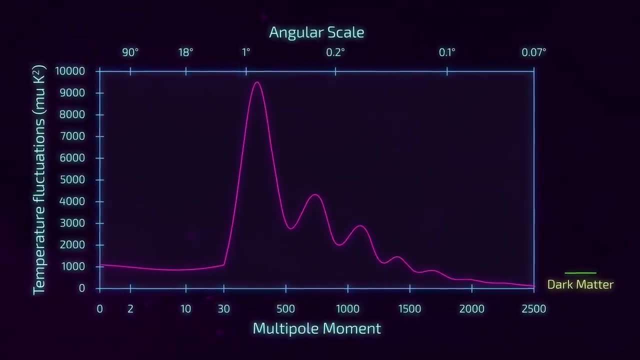 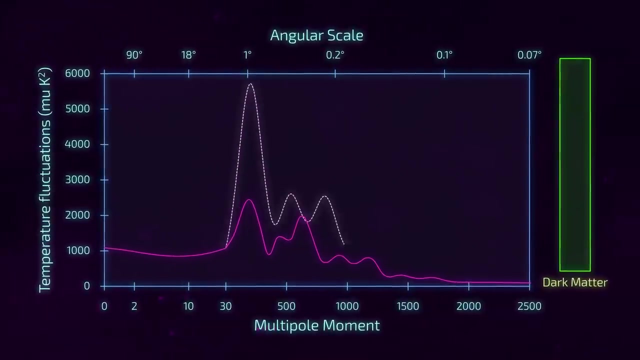 of decreasing size. Now, the height of these peaks depends on how much dark matter there is. In a universe without dark matter, the graph looks like this, But as dark matter increases, the amplitudes of even-numbered peaks decreases To match the measurements of the CMB. 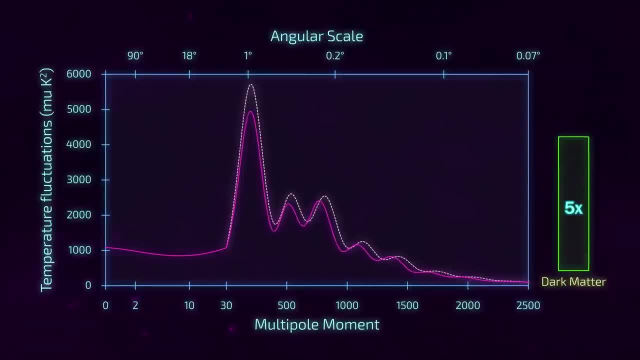 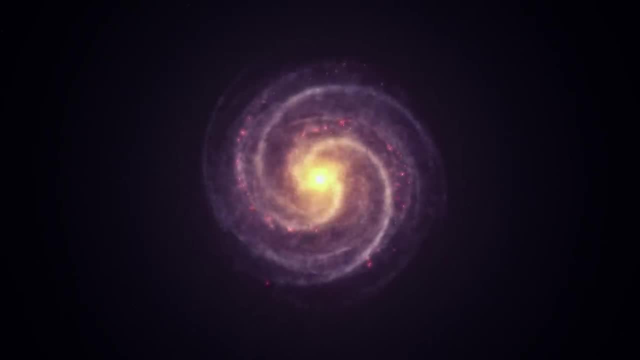 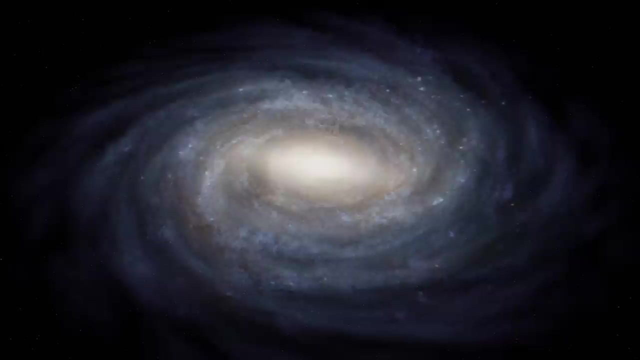 we need about five times as much dark matter as ordinary matter. This figure also agrees with the amount of dark matter required to explain the motion of stars in galaxies and the motion of galaxies in clusters. So the dark matter hypothesis explains a lot of different observations. 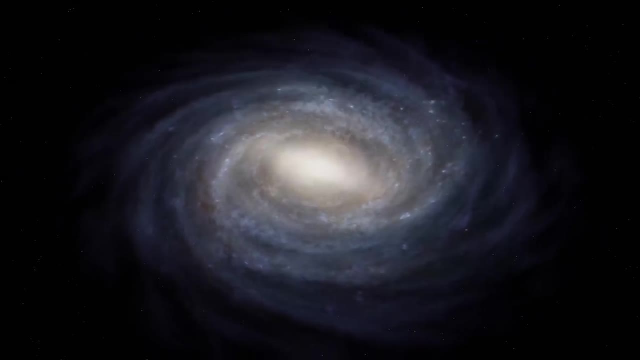 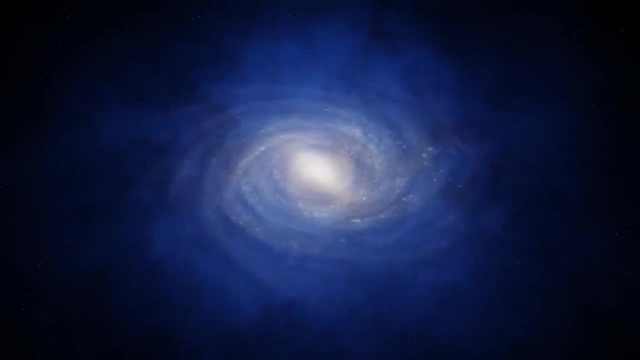 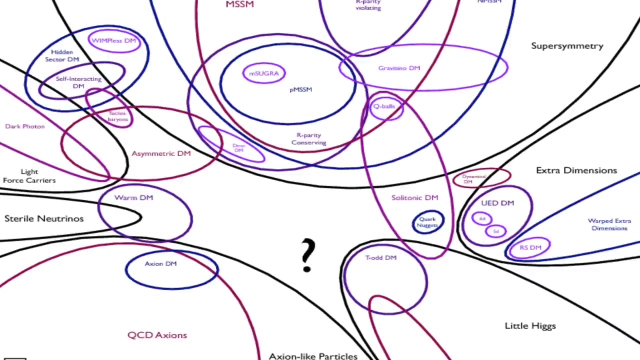 with a simple theoretical framework: that there's some type of particle out there that only interacts through gravity. But what is this particle exactly? Since we don't know, scientists have proposed a whole bunch of different things that it could be, and now we have to try to go out and find them. 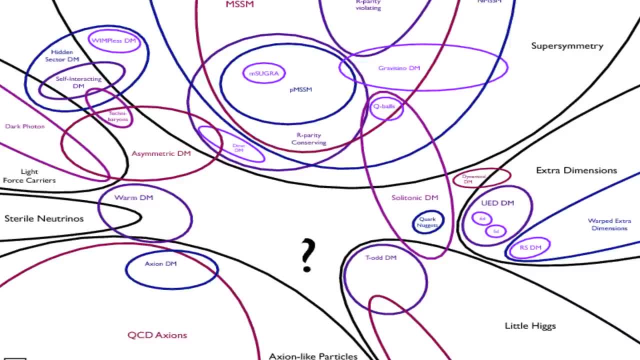 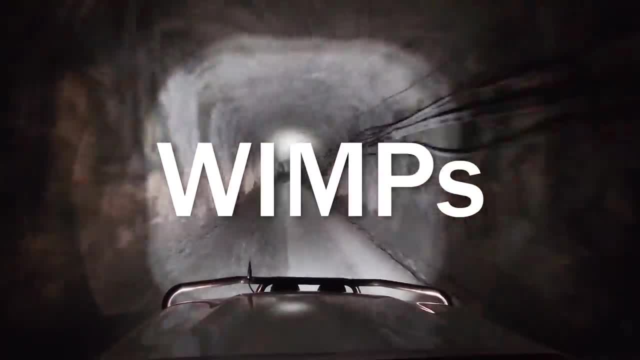 The approach differs depending on what you're trying to find. Dama Libra and the detector at the bottom of the goldmine are looking for WIMPs, Weakly Interacting Massive Particles. These particles are expected to weigh about as much as a proton. 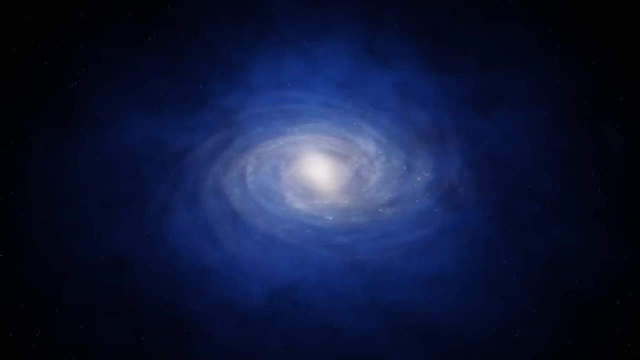 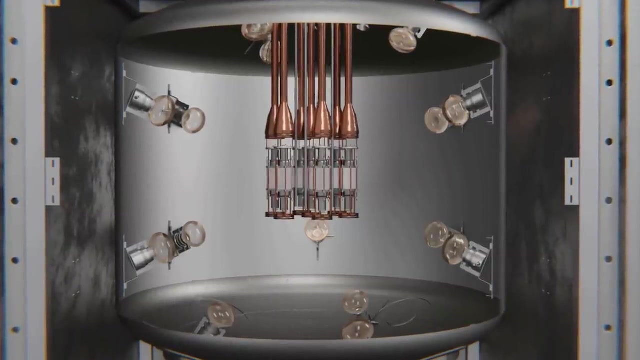 but interact with ordinary matter extremely weakly. At the heart of the detector are seven 7-kilogram crystals of pure sodium iodide. So that's actually sodium iodide in there. Yep, I didn't expect it to be so clear. 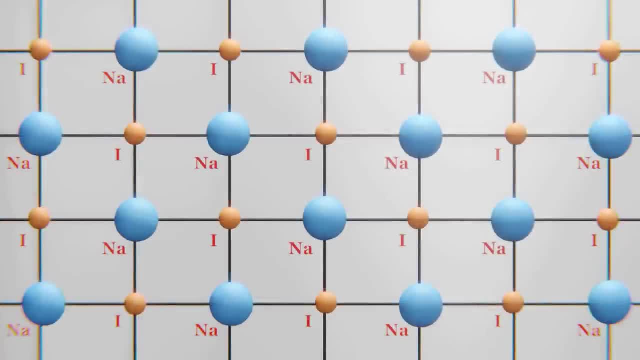 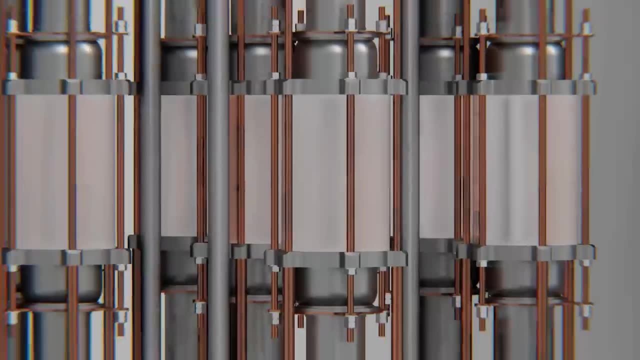 The idea is that very, very rarely a dark matter particle may hit a nucleus in the crystal and transfer its energy. This creates a flash of light called a scintillation, which is detected by photomultiplier tubes, very sensitive light detectors. 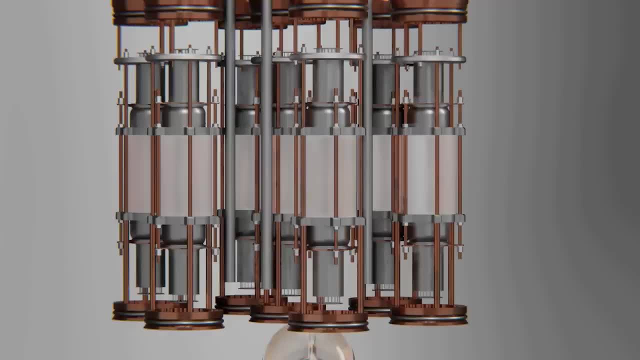 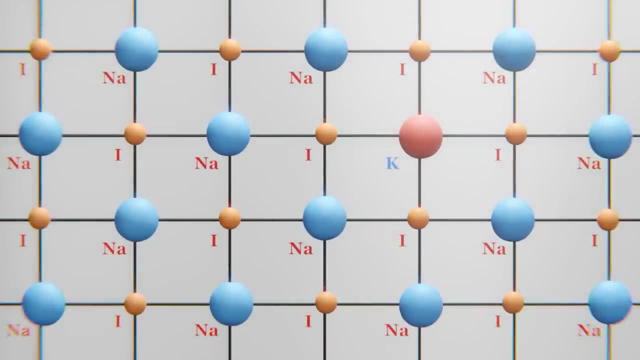 which are positioned above and below each crystal. But there's a problem. Even the purest sodium iodide crystal contains radioactive potassium, and when a potassium atom decays, it emits an electron and a gamma ray. Now the electron can cause a scintillation. 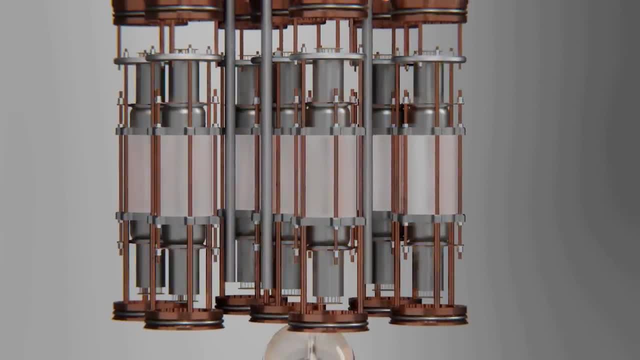 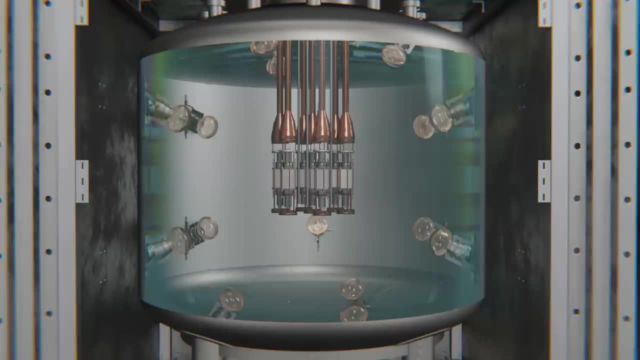 in the crystal, just like the hypothesized dark matter particle. So, to eliminate these events, the sodium iodide crystals are submerged in a tank full of 12 tons of linear alkyl benzene. This is a liquid scintillator that emits light. 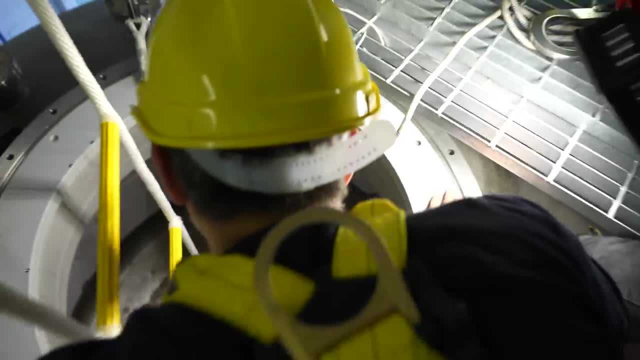 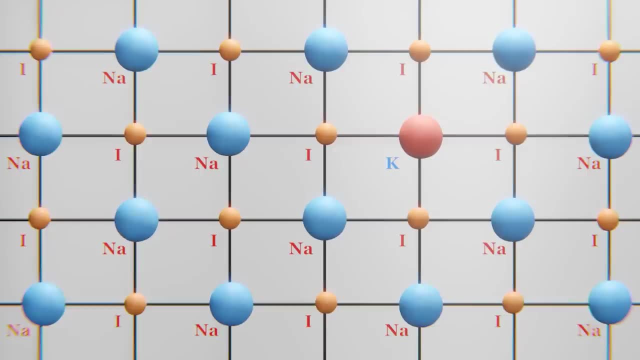 when exposed to a gamma ray, And that light can then be detected by photomultiplier tubes in the tank. So if there's a simultaneous detection in the crystal and in the tank, it was most likely a potassium decay, not a dark matter event. 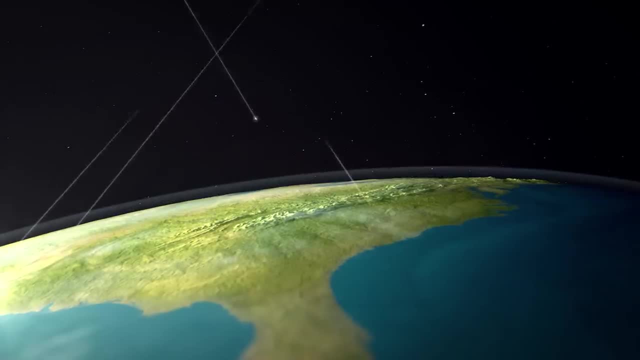 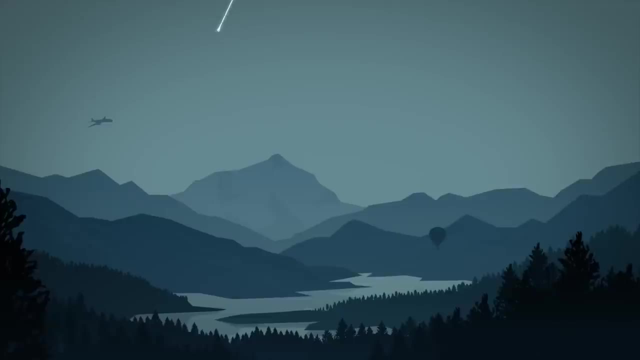 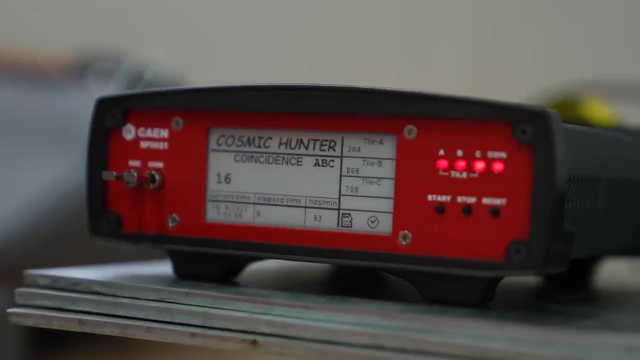 But there's another problem. This is a muon detector and it's got these three paddles of plastic here, separated by some pieces of steel. If we see a flash of light in all three, basically at the same time, then it's a muon detector. 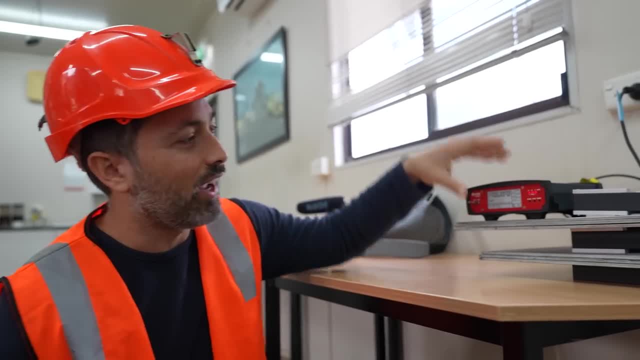 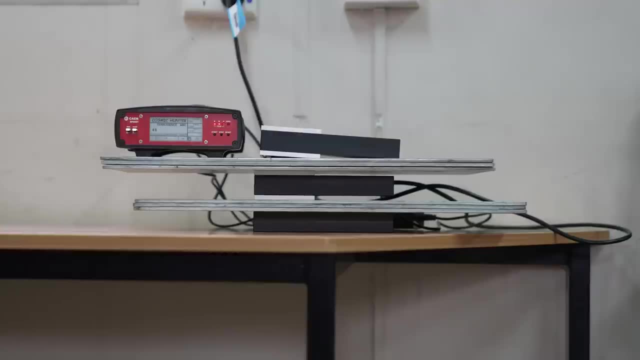 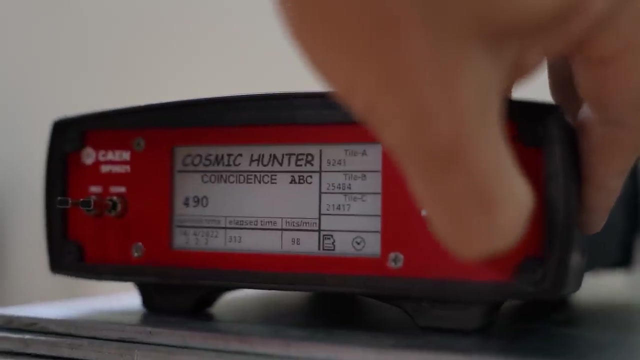 And the muon detector can detect light in the same time. So the muon detector can detect light in the same time, in all three basically at the same time, then we know that a muon has passed through them. So if I hit reset. 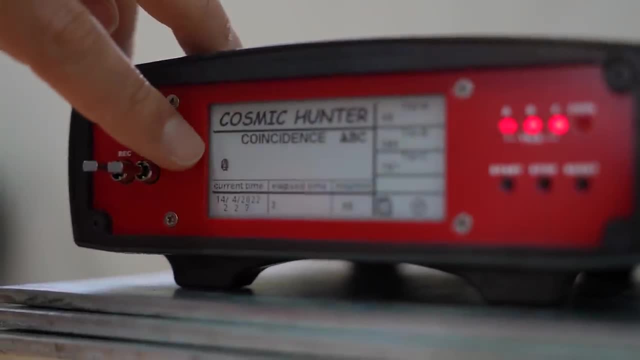 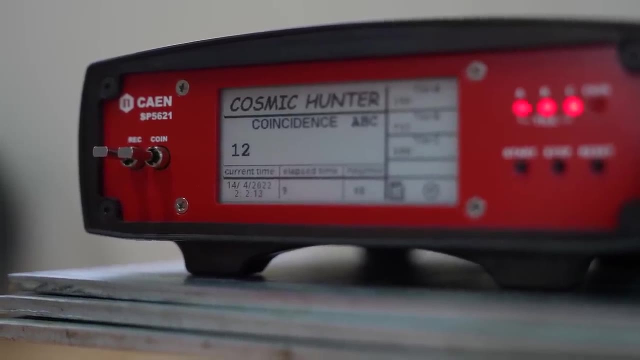 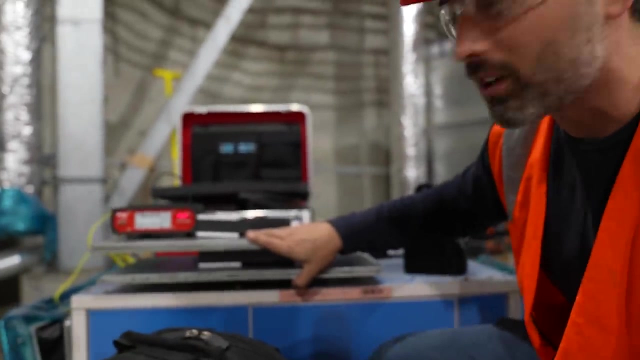 we can see counting up the muons being seen, so it's at least a few a second. This is why all sensitive particle detectors are located deep underground. Here we have the muon detector now one kilometer underground. It's been running for something like: 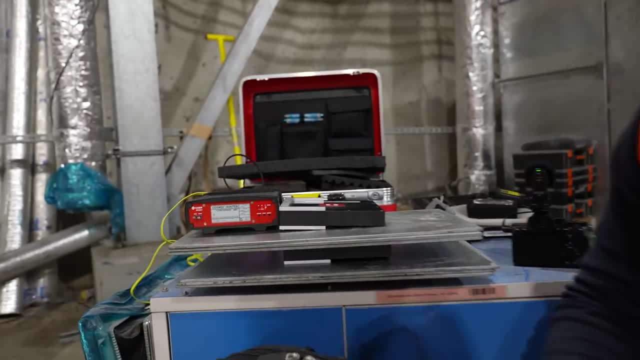 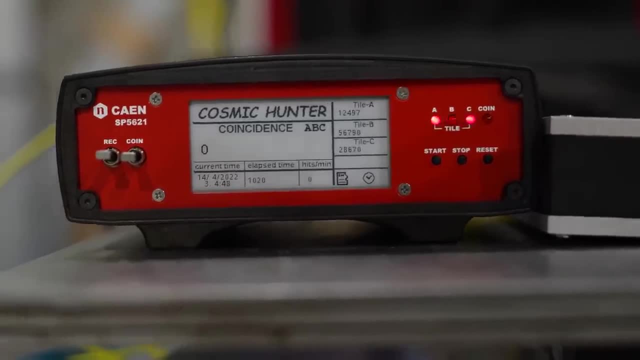 15 minutes and there have been no muon counts. Yeah, we'd have to leave this running for a long time, I think, even if we wanted to get a single hit. We expect the number of muons down here to be about a million less. 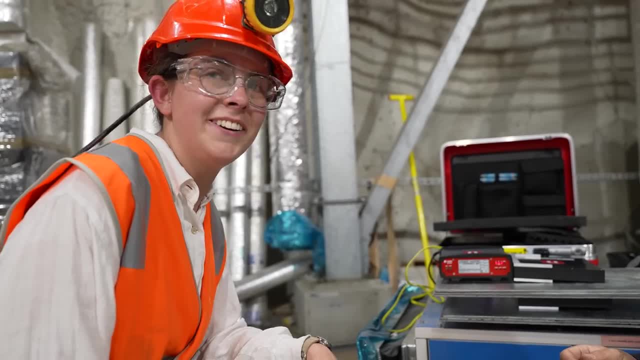 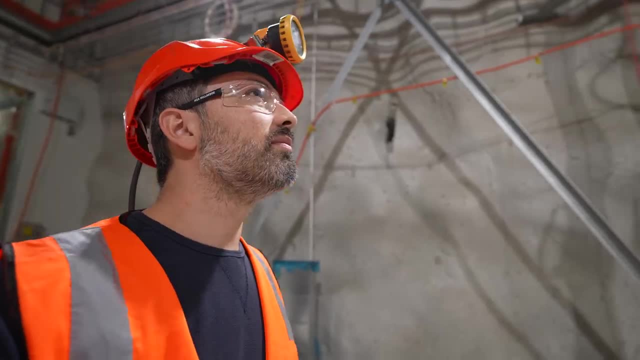 And we didn't see a million at the top, so we're probably not going to see any down here. And this is the whole point of putting a dark matter detector underground: You want to get rid of all the background that would create noise in the detector. 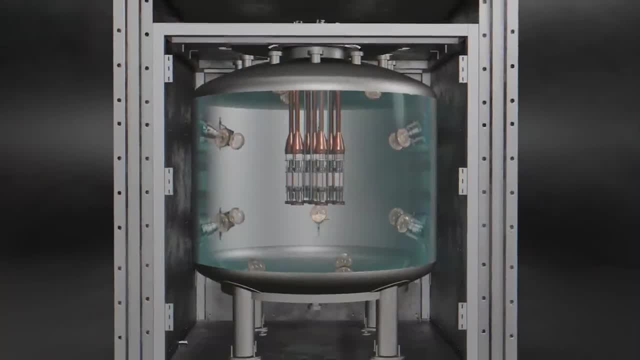 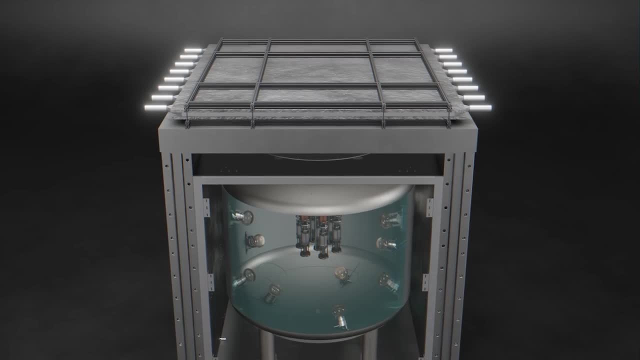 But even this shielding is not enough. They'll have muon detectors immediately above the tank, so if a flash is seen in a crystal, at the same time a muon is detected it can be ruled out. Being underground brings its own challenges. 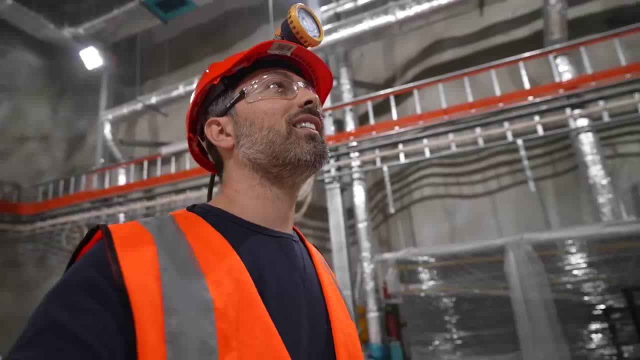 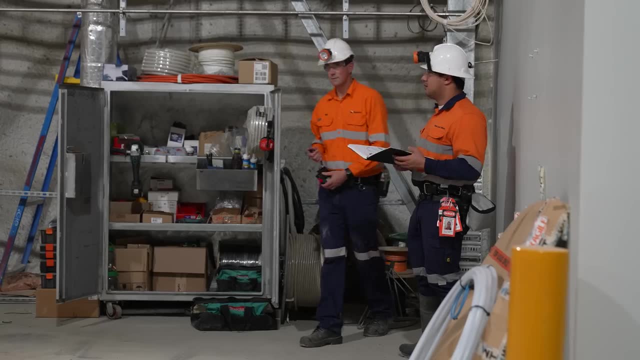 The walls of the mine contain trace amounts of radioactive elements like uranium and thorium, which decay into radon gas. The requirements here are fairly serious. for a dark matter experiment, We have to completely control the environment, in particular the radon level. 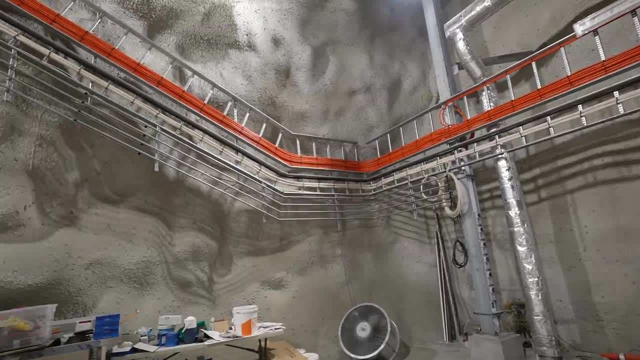 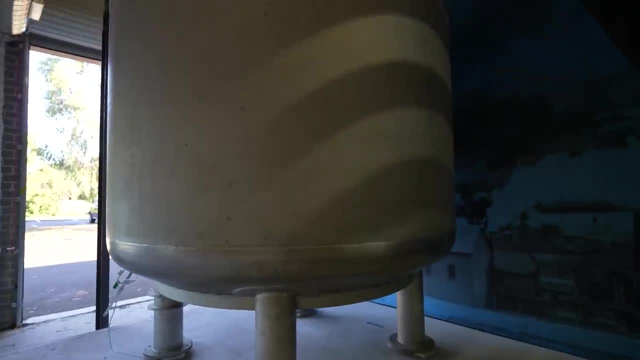 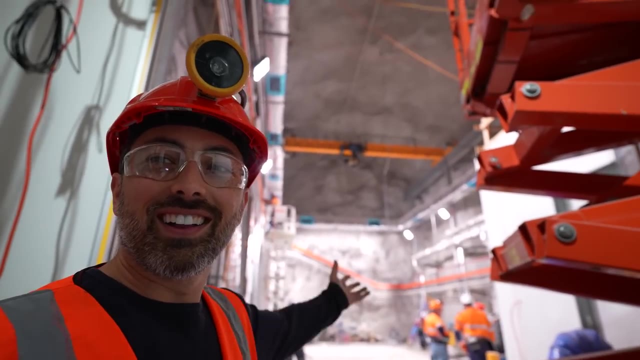 To counteract this, the walls of the cavern are coated with special paint to contain radioactive particles, They are immersed in a continuous stream of pure nitrogen gas, And the entire detector is shielded by 120 tons of steel and plastic. Wow, Look at the size of that cavern. 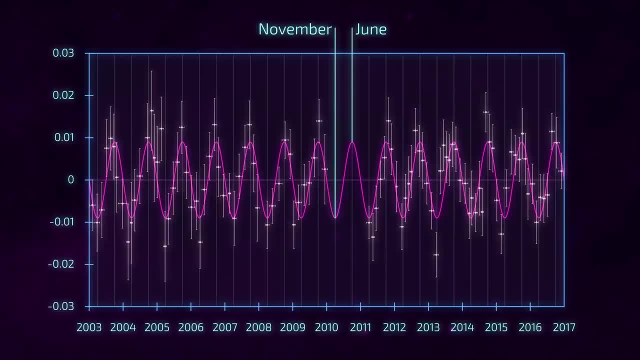 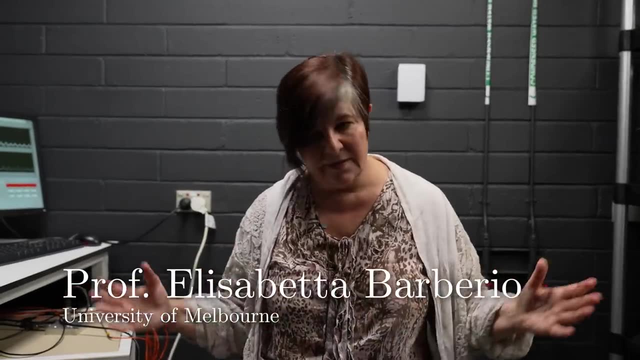 There is a lot riding on this experiment. It will validate or disprove one of the most contentious results in physics. So if we see nothing well, this is the dead of Dama Libra. But if we see something well, we are all happy. 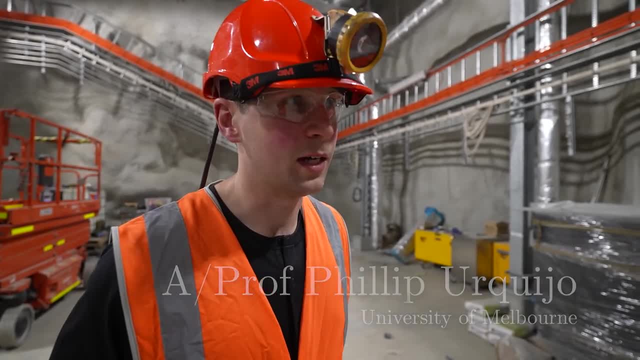 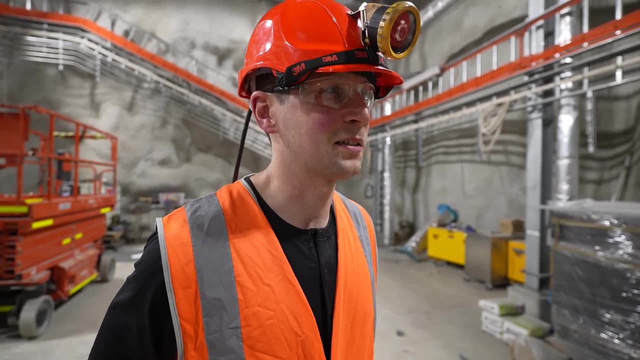 I like the idea that, because 80% of the mass of the universe is dark matter or dark stuff, maybe there is more than just one particle that dark matter is made of. It could be an entire dark standard model, a dark version of everything that we can see. 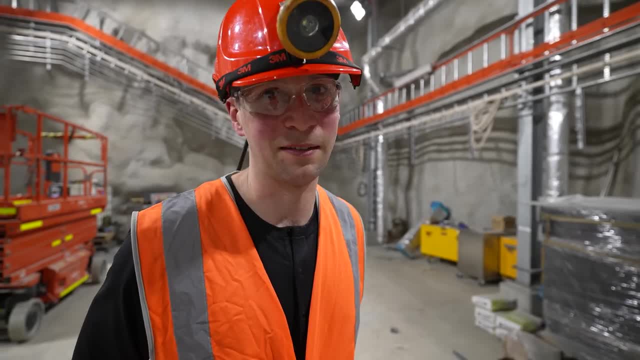 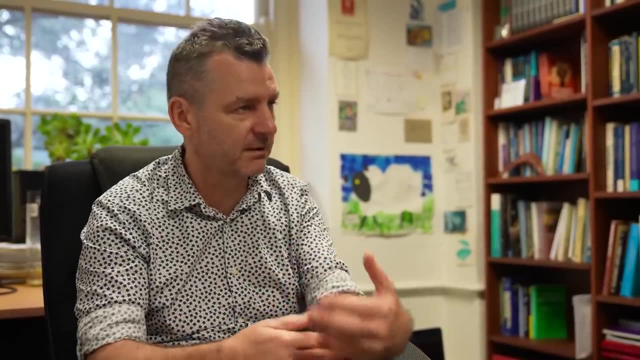 or maybe something more complex, because there is so much more of it. I really hope it's that. Do you think that dark matter interacts with ordinary matter? If we want to find out what this stuff is, we better hope there is some level of interaction. 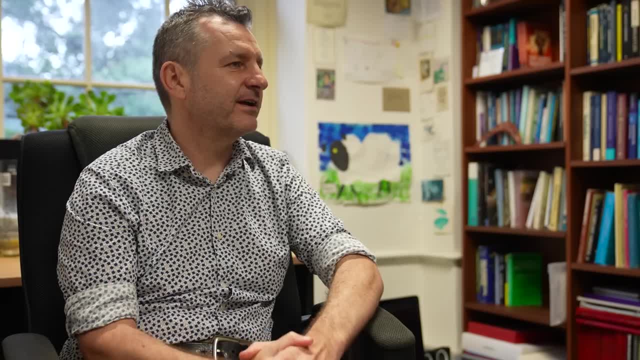 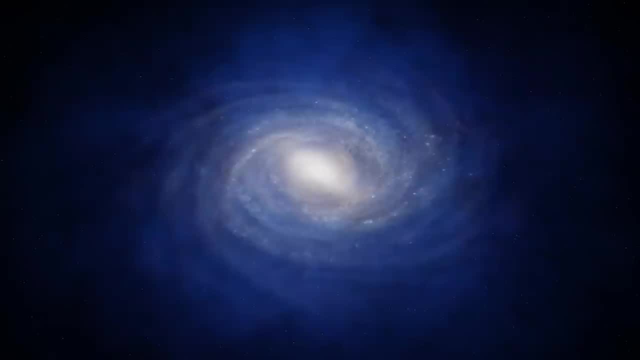 that we can at least probe when it comes to doing experiments. If God gave me the great book of physics and there were two sections, section A and section B, one for the luminous matter and one for dark matter, and they didn't talk to each other. 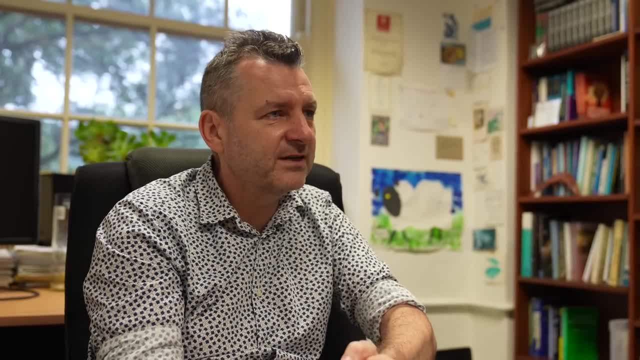 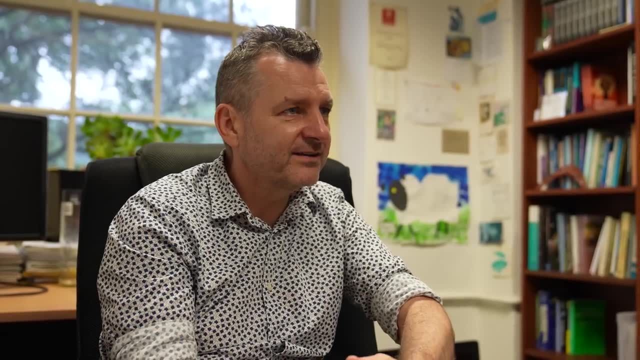 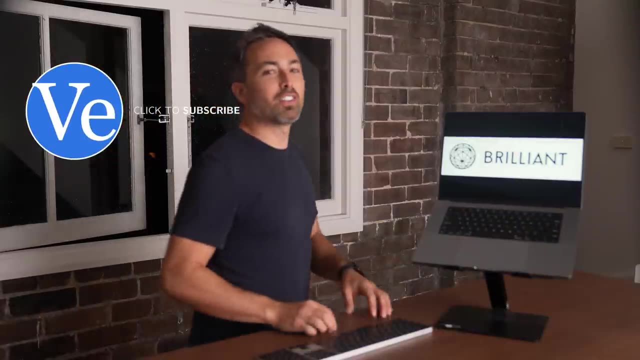 I would say that was a very peculiar universe. But in science we have to live with the possibility that at some level we may never find the answer. It may elude us, but at least we tried. The sponsor of this video: Brilliant is the opposite of dark matter. 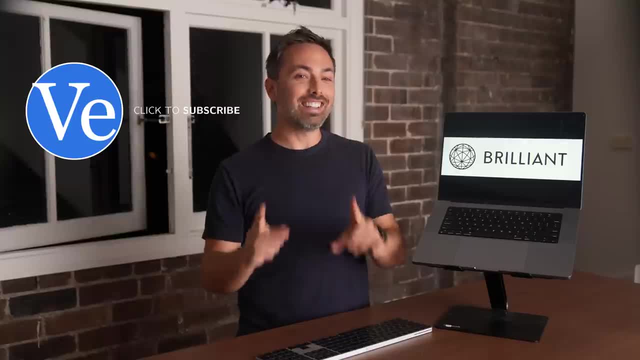 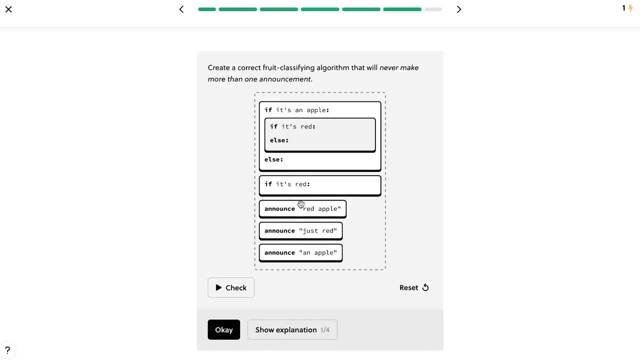 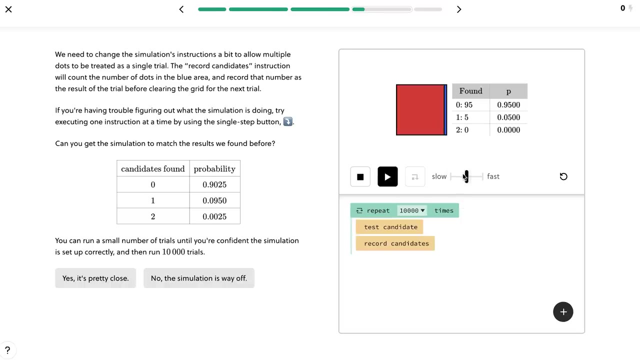 You see it everywhere and it's highly interactive. Brilliant is an innovative STEM learning platform that guides you through engaging, hands-on courses in math, science and computer science. They have great courses on so many topics, from pre-algebra to probability to computer science fundamentals. 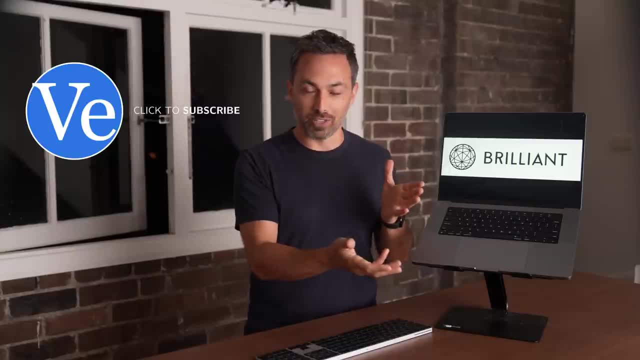 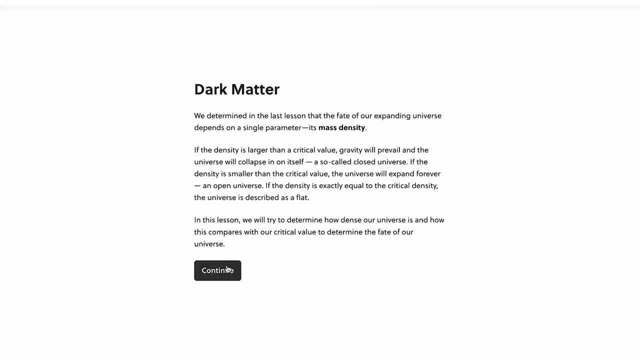 It's the ideal complement to watching educational YouTube videos. After learning about a topic, you can dive deeper and get your hands dirty and really understand it, For example, if you want to learn more about dark matter, gravitational lensing and the cosmic microwave background. 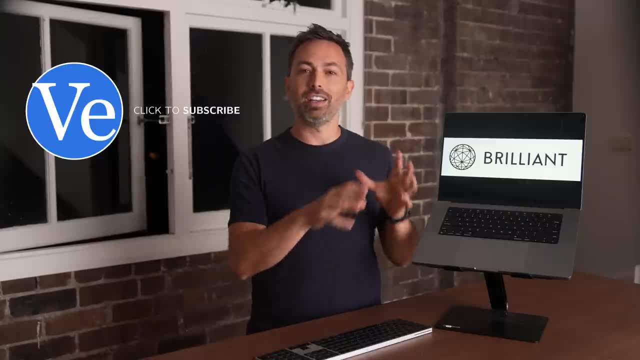 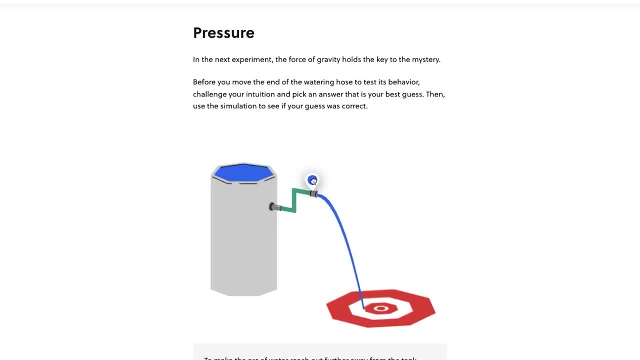 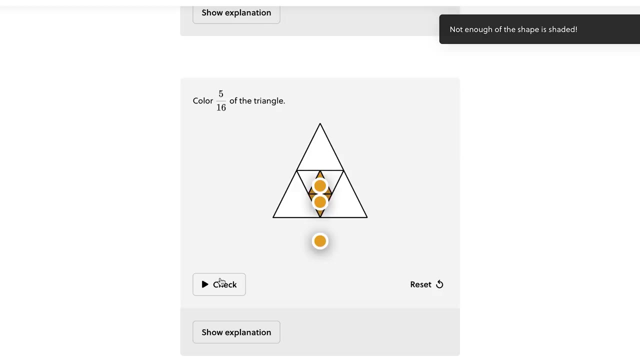 I highly recommend their astrophysics course. A lot of care and attention goes into all their courses. Every lesson and interactive simulation builds on what you've learned previously And every step of the way your knowledge is tested through quizzes which check your understanding and reinforce what you've learned. 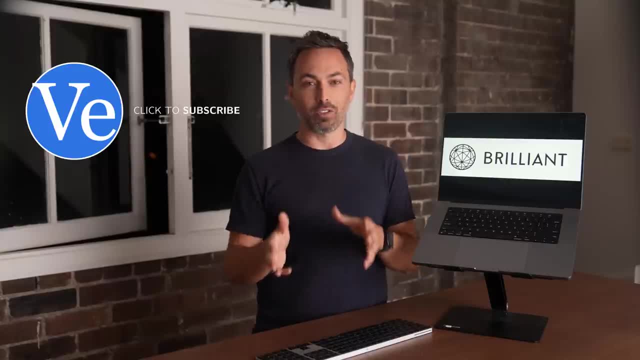 If you get stuck, there's always a helpful hint, So I encourage you to check out the courses on offer over at brilliantorg slash veritasium, And I bet you'll find something there that you want to learn more about, Plus if you click through right now. 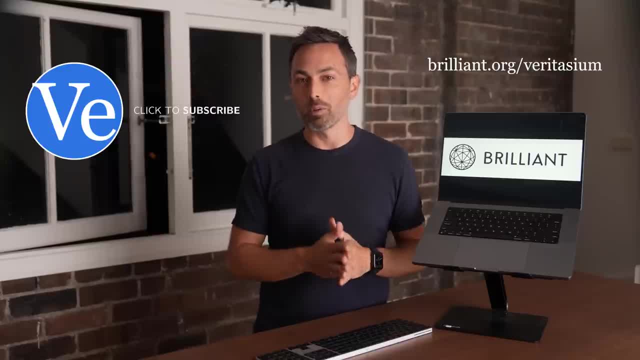 Brilliant are offering 20% off an annual premium subscription to the first 200 people to sign up. So I want to thank Brilliant for supporting Veritasium and I want to thank you for watching.